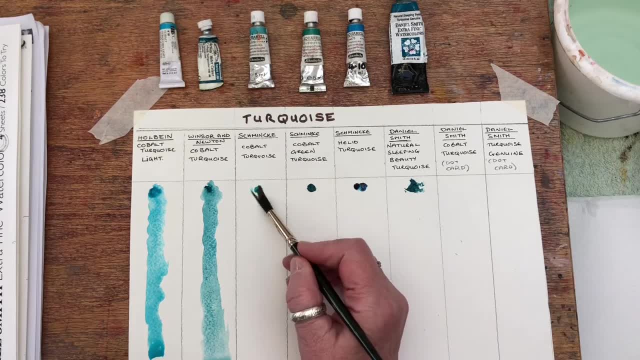 This one is the Schmincke, Tinted. This is by Winsor & Newton. This is by Winsor & Newton. It's a bit darker but still works fine once you get it re-wetted. a cobalt turquoise. You can always see that some of these are a bit easier to. 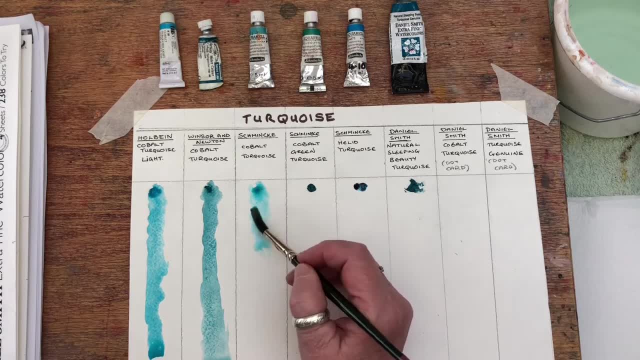 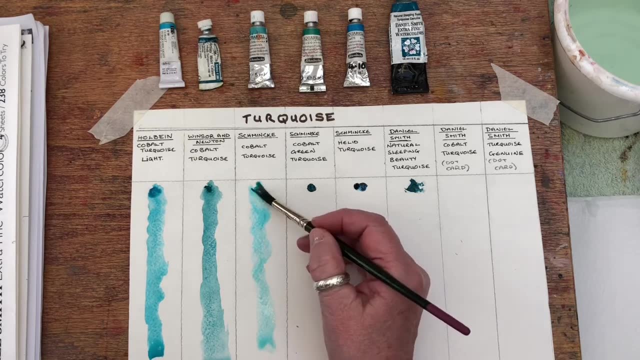 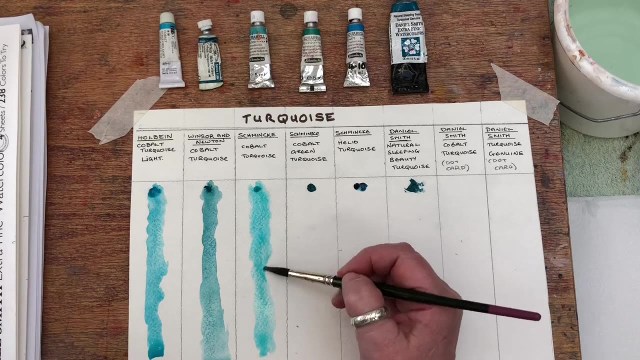 wet than others. Okay, it's a pretty colour. another pretty colour: yep, Slightly paler, kind of baby blue. I might call that really A little bit similar to this one. This one, I'm expecting to be a little bit different, because this is the 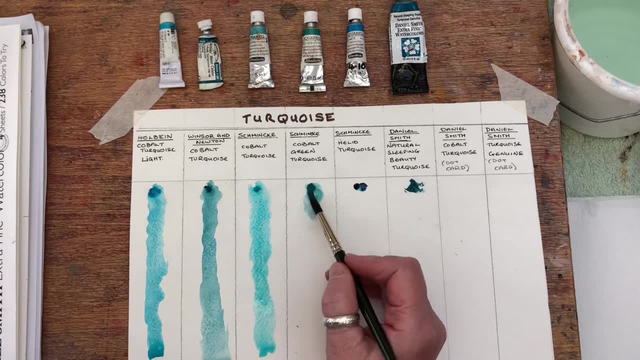 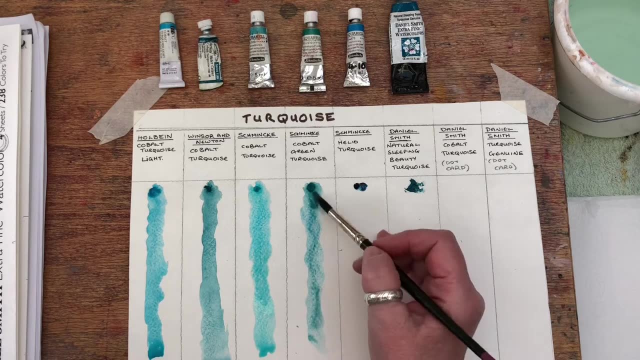 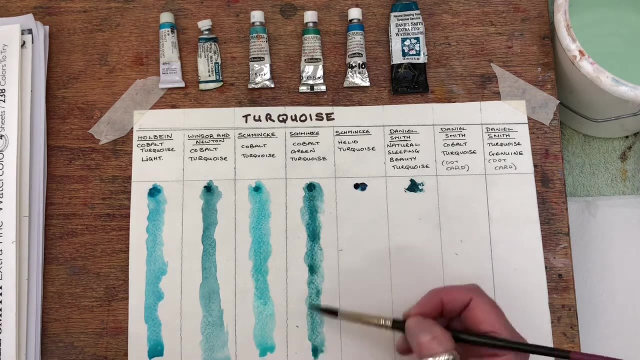 Schmincke: cobalt green turquoise. Is it different? Let's have a look. Not too different really If we compare it with this one, the Winsor & Newton Interesting. I think that would make a nice sea colour. turquoisey green sea colour. 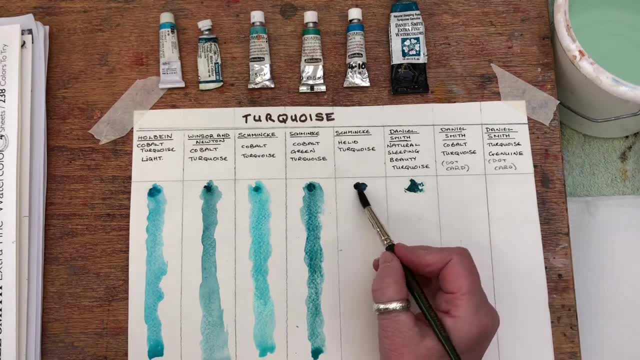 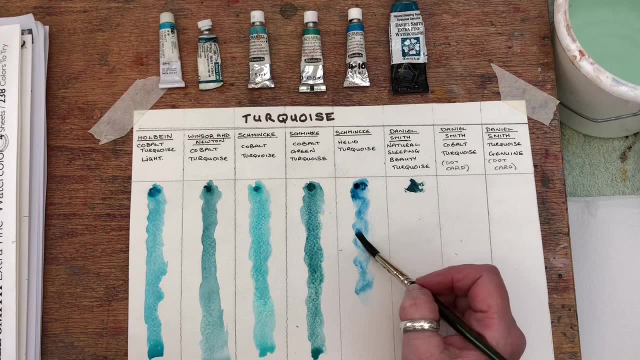 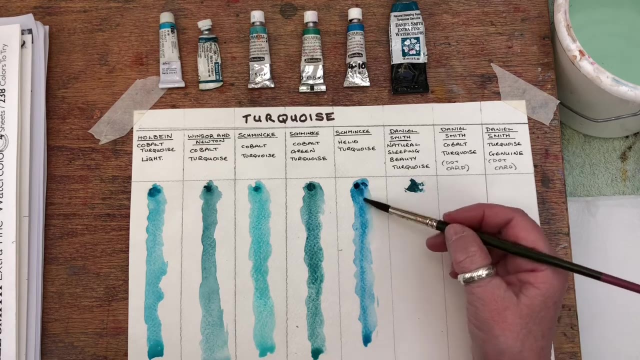 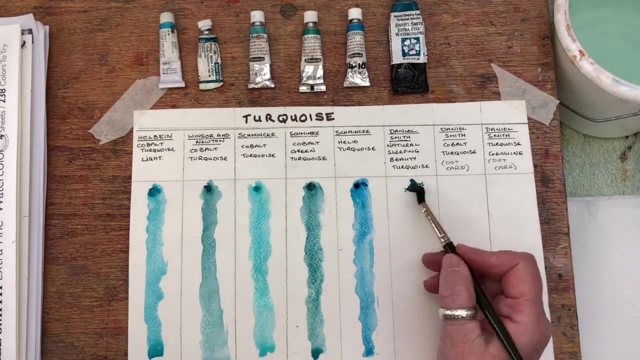 This one's one of my favourites: Schmincke Helio turquoise. I find this one very pretty. Swimming pool blue. I call that Lovely um. this one is the Daniel Smith natural sleeping beauty turquoise, which is a brilliant name, isn't it Very romantic? natural sleeping beauty turquoise. 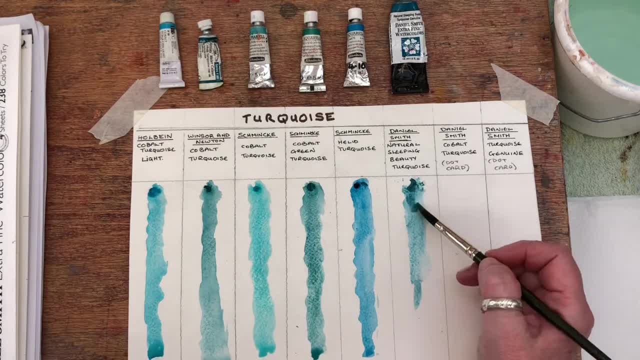 I don't think this only comes in the larger Daniel Smith tubes- don't quote me on that, but I think so- The 50ml tubes, which obviously makes it a bit more. then, to be honest, much more than that. That's lovely, lovely Campbell's ball painted turquoise. 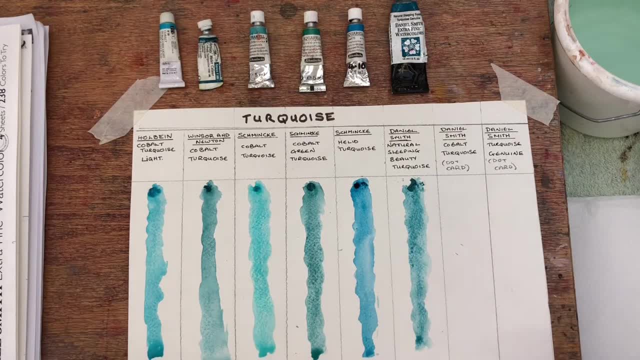 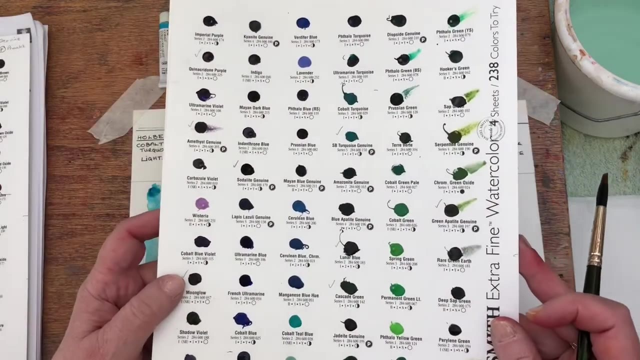 expensive if you want to invest in that Right. these last two, these Daniel Smith Cobalt Turquoise and Turquoise Genuine- I'm going to take off of the Daniel Smith dot cards because at the moment I don't have tubes of these, but I'm interested to see what they do, what they look like. 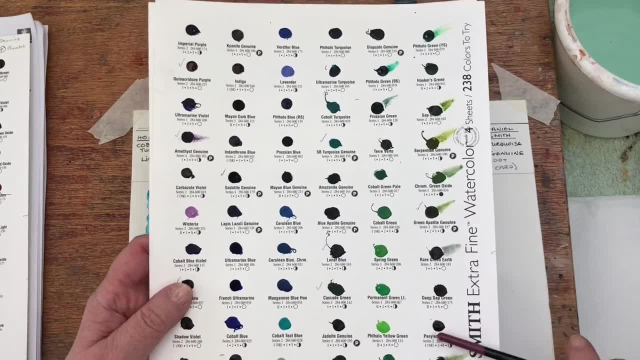 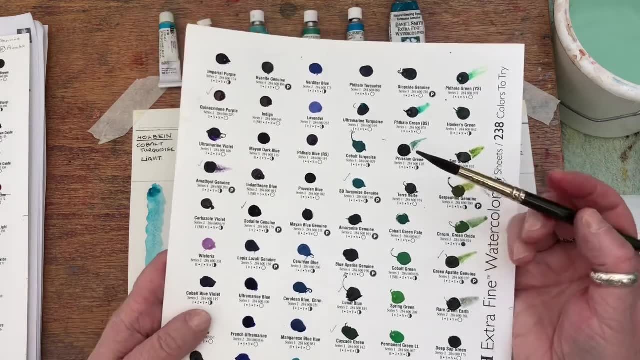 So Daniel Smith sell these watercolour dot cards which you can buy, and there's four or five all together with different colours on. This is the sheet that happens to contain some of the greens and blues turquoises, So this one is Cobalt Turquoise. all you have to do is just 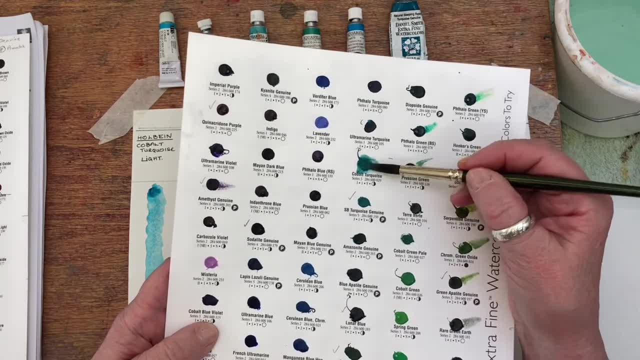 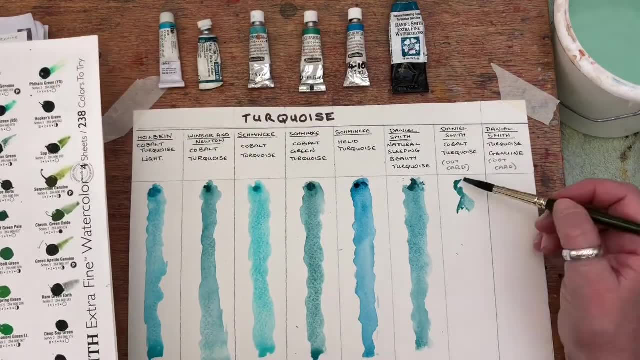 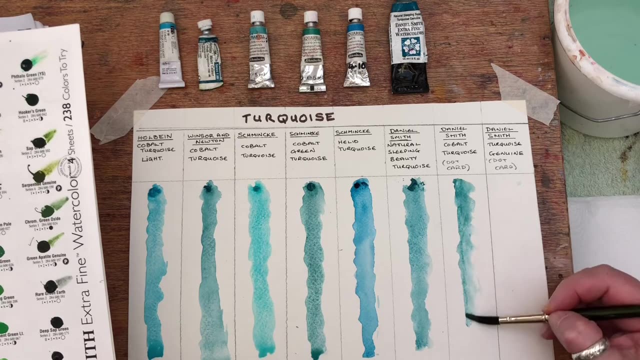 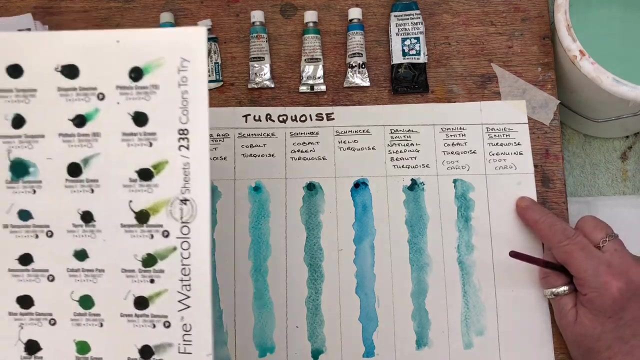 dump your brush and lift it from the dot card. There's little amounts of paint on here from the tube. So this is Cobalt Turquoise And the last one is the Daniel Smith Turquoise Genuine, which is this one on the dot card. 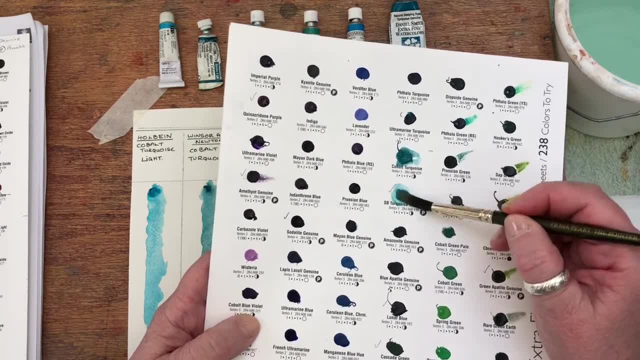 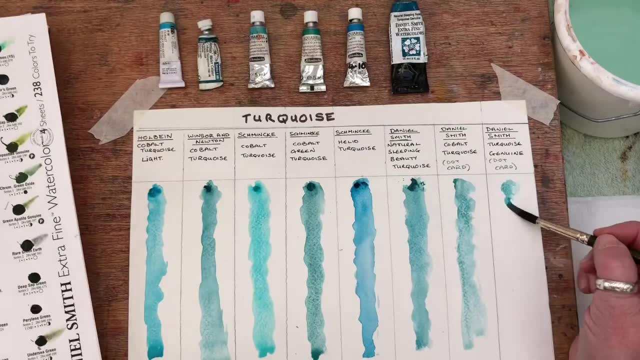 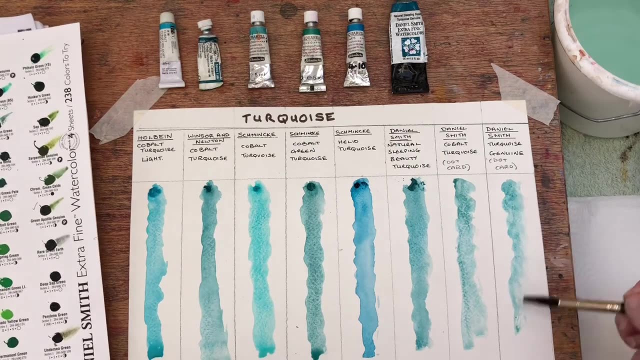 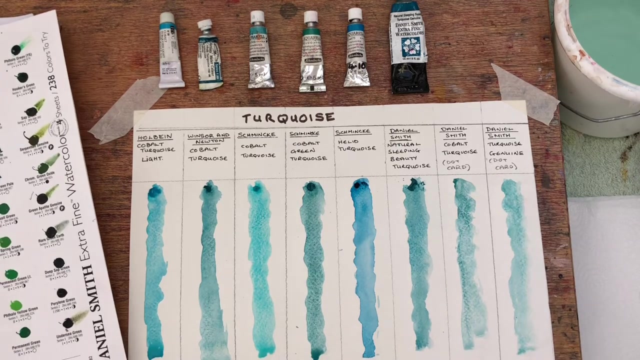 Interesting to see how much difference there is between these two. That should be enough. A little bit more, Okay, the Daniel Smith Turquoise Genuine. A whole array there of different turquoises and you can also see how some of them are granulating more than others. I mean, most of them are granulating. 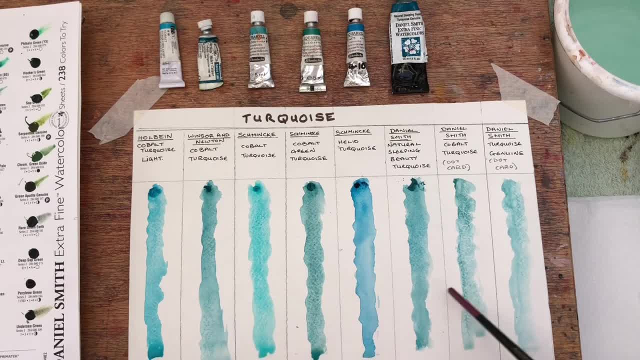 The Schmincke Helio Turquoise, that hasn't really granulated. Not much evidence of that granulating. The Daniel Smith ones are granulating a lot, actually Particularly this one that's very pretty, Imagine that one for being kind of a sea turtle. 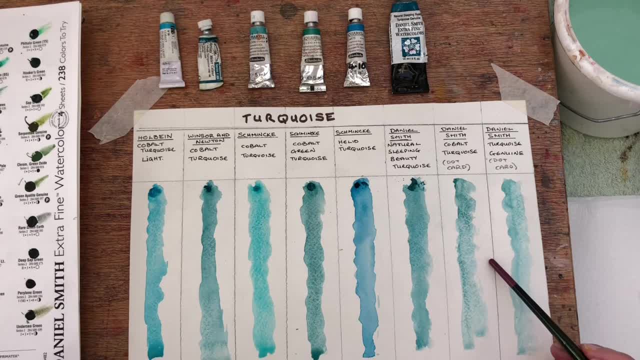 I don't know if you can see it, but it's a sea turtle. I know the Helio Turquoise is very transparent. The others I'd have to check- Semi-transparent, it looks like for these two, Which is interesting. If I look at the back of the Schmincke, it should tell me. 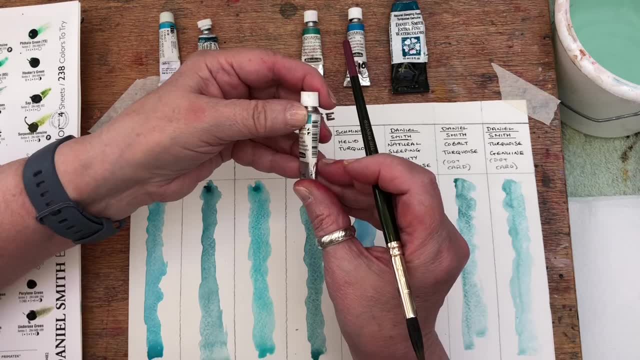 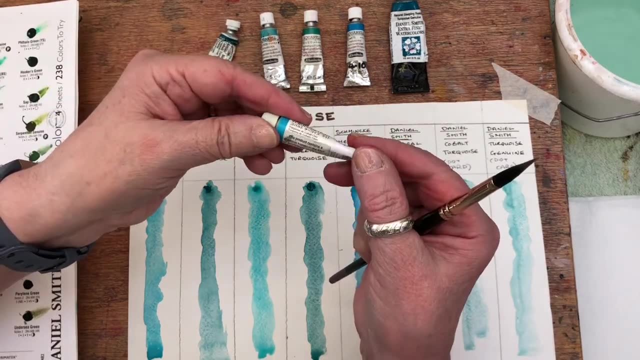 You can do your own studies. of course, Semi-opaque this one, the Schmincke, I don't always tell you on the tube, unfortunately, so you could refer to my other video on this channel, which tells you all about how to find out.